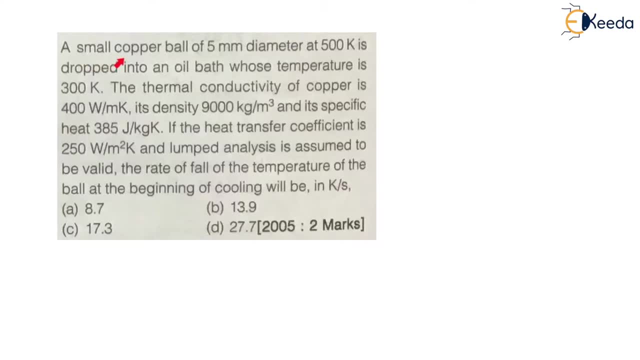 So let us understand the question. The question is a small copper ball of 5 mm diameter. Now here, copper ball is given. Therefore ball is always spherical. Therefore the given object is a sphere, copper sphere, Right. And it is a ball means it is a sphere And diameter of sphere is given 5 mm. 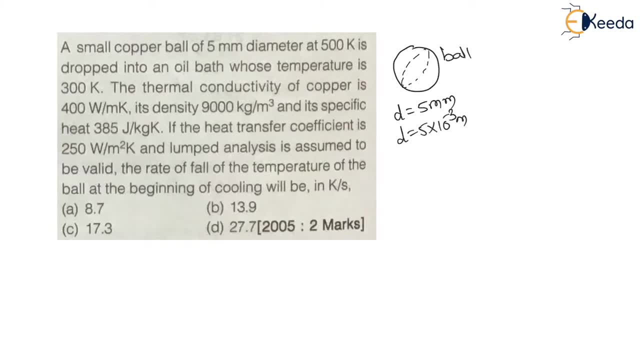 Therefore I can say: diameter is equal to 5 into 10, to the power minus 3 meter in terms of meter. Then a copper ball of 5 mm diameter at 500 Kelvin. Now it is at 500 Kelvin means initial temperature of this ball is Ti. 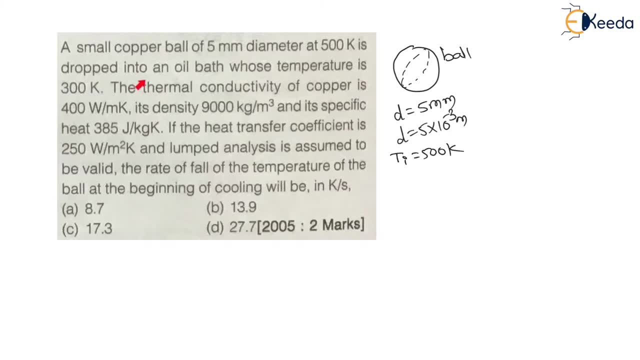 Which is 500 Kelvin Right, Is dropped into an oil bath whose temperature is 300 Kelvin. Now oil bath is nothing but surrounding fluid. Therefore, this surrounding fluid temperature is nothing but T infinity, Which is 300 Kelvin Right. Then the thermal conductivity of copper is 400 Watt per meter Kelvin. 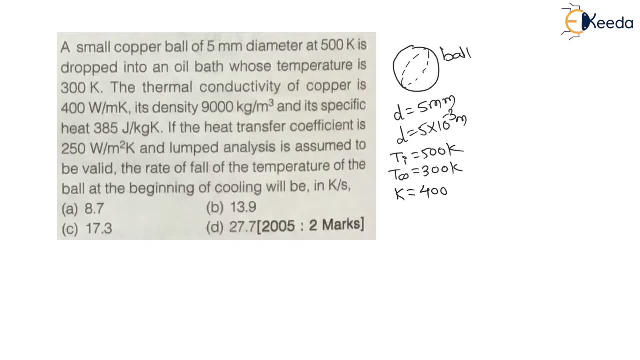 Now here thermal conductivity of copper is given, which is 400 Watt per meter Kelvin, Then Its density. Density is given 9000 kg per meter cube. Therefore rho is equal to 9000 kg per meter cube. Then And its specific heat, that is Cp. 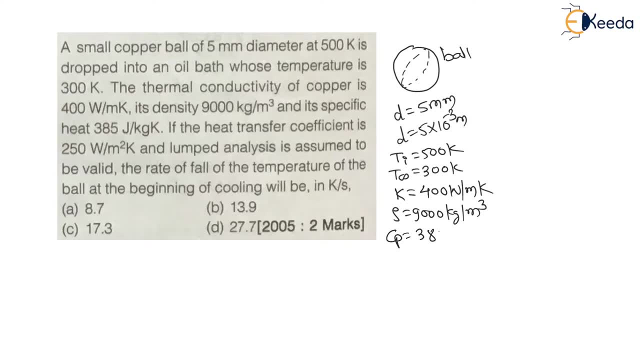 Specific heat Cp is given, which is 385 Joule per kg Kelvin, Then If the heat transfer coefficient is 250 Watt per meter square Kelvin, Heat transfer coefficient is nothing but convective heat transfer coefficient, which is, Eh It is given 250 Watt per meter square Kelvin. 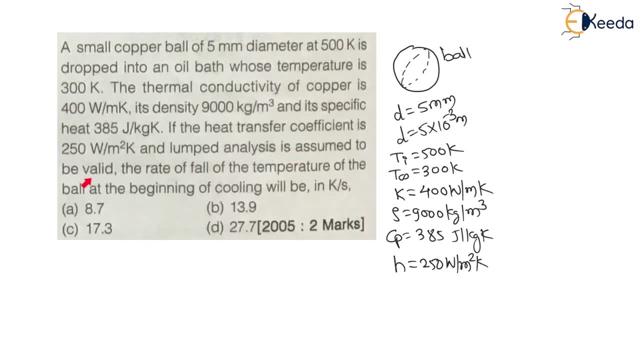 Then, And lumped analysis is assumed to be valid. Very important, My dear students. Here they are saying The lumped analysis is assumed to be valid. means we can use the formulas of lumped analysis. The rate of fall of temperature of the ball at the beginning of cooling will be in Kelvin per second. 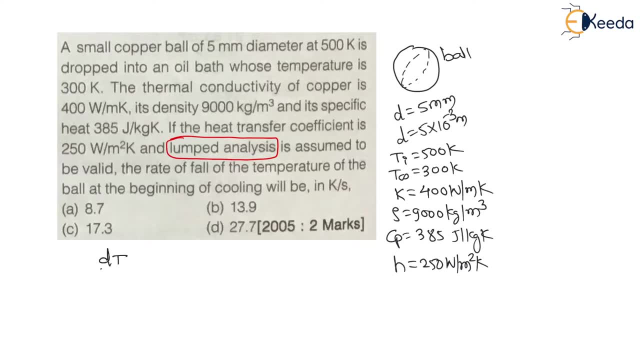 Now they are asking The rate of fall of temperature, That is, Dt With respect to time. Dt by Dt, Right At the beginning, will be At the beginning of cooling Means whenever time is equal to zero. Right, They are asking change in temperature with respect to time when time is equal to zero. 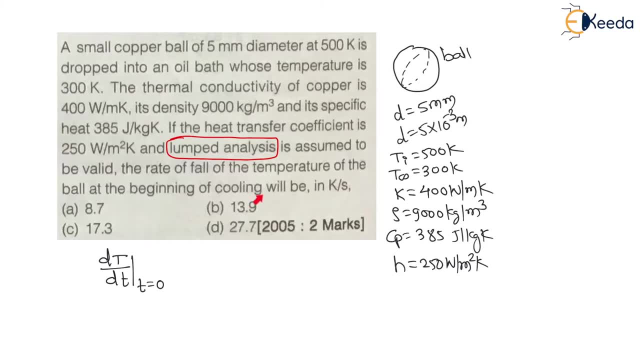 That is called rate of fall of temperature at the beginning of cooling will be in Kelvin per second. This is the question Right Now. my dear students, Let us solve this question Now. I will tell you: the answer is option C. For this question, the option C will be the correct choice. 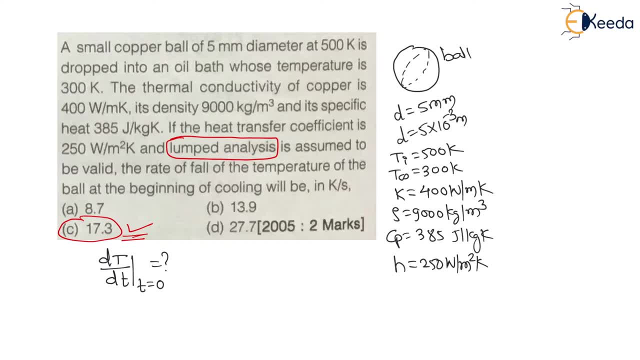 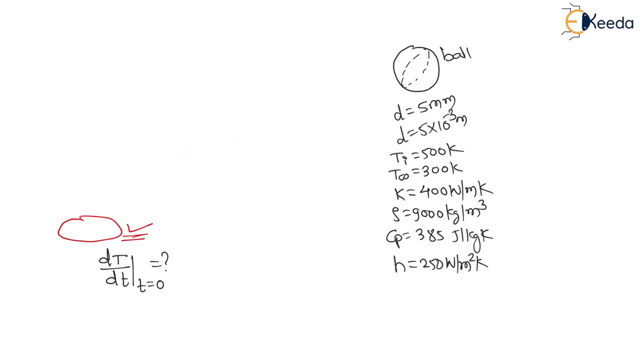 Right Now. let us pause the video and solve this question Now. here I am going to delete this question, So that will get sufficient space for the solution Now. let us solve this question Now. my dear students, Here They are asking rate of fall of temperature. 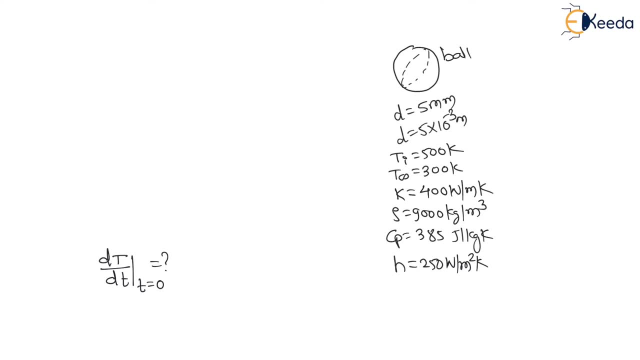 That is Dt by Dt. Now for this lumped capacity analysis, or lumped analysis. we have derived one formula that is temperature at any instant of time minus surrounding fluid temperature. They have an initial temperature. minus surrounding fluid temperature is equal to e, to the power. 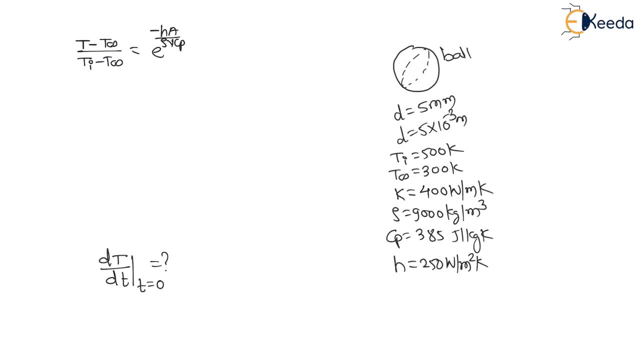 minus H A, divided by rho, V, C, P into T. That formula we have derived. But they are asking to find DT by DT. So let us find this temperature equation. Therefore we can say T minus T infinity is equal to T I minus T infinity. 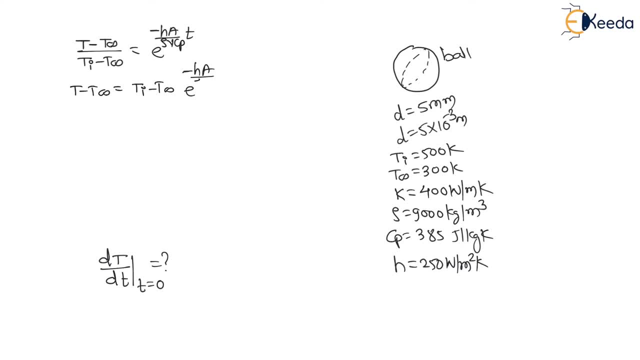 into e to the power minus H A divided by rho V, C, P into T. Therefore, we can say: this temperature profile will be equal to T infinity plus T, I minus T, infinity. e to the power minus H A divided by rho V, C, P into T. Now here, 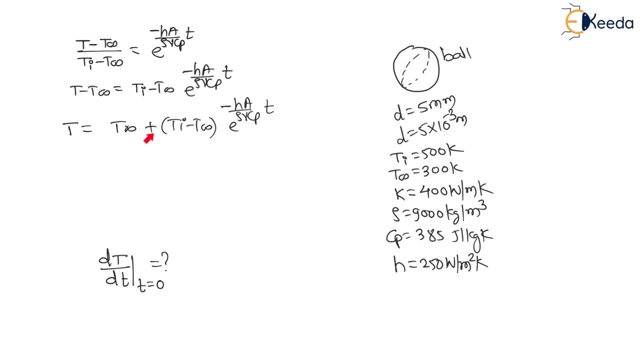 change in temperature with respect to time. we have to calculate. So let us differentiate this equation. If I differentiate this equation, I will get DT by DT with respect to time. We have to differentiate with respect to time. The surrounding fluid temperature is always constant, Therefore derivative. 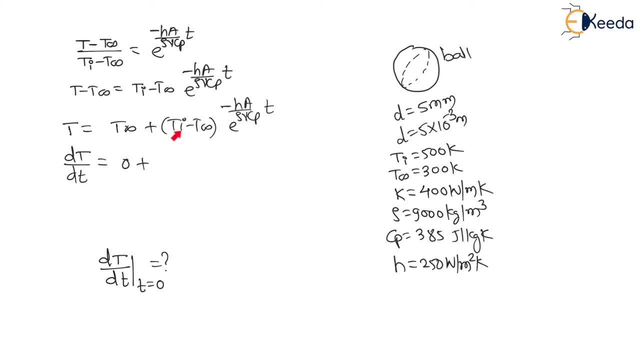 of constant is 0. Plus now this wall, initial temperature is always constant. Initial wall temperature and surrounding fluid temperature is constant. Therefore, we can write T, I minus T, infinity. Now e to the power. What will be the derivative of this? 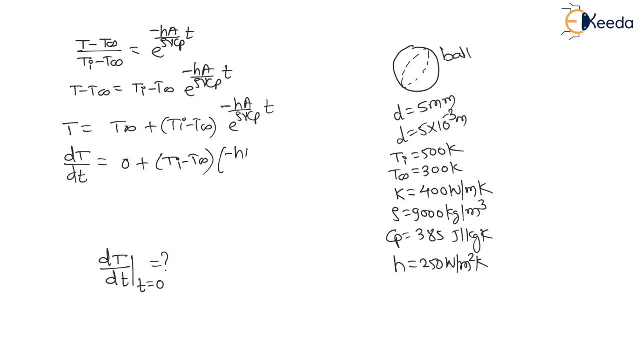 This factor will come out: That is minus H A divided by rho V C P. This factor will come out And this power will remain as it is. That is e to the power minus H A, divided by rho V C P, into T. 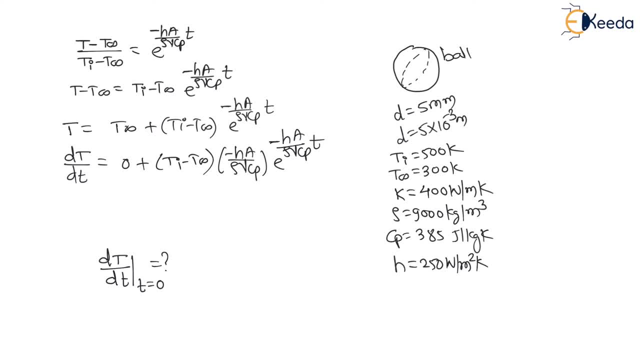 This will be our final resulting equation. Now, my dear students, here we have to find this rate of fall of temperature with respect to time, when time is 0.. At the beginning of cooling. They have mentioned at the beginning of cooling. Therefore, we have to find this DT by DT. 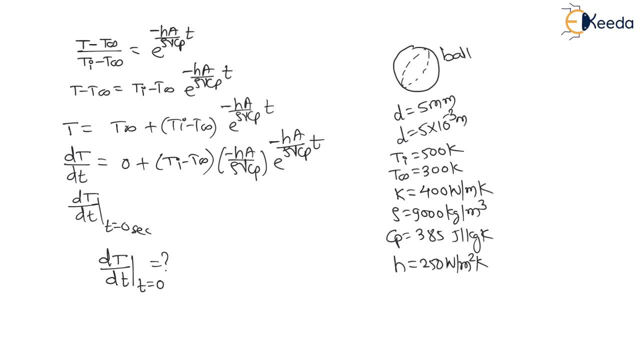 when time is equal to 0 second. So let us put this: T is equal to 0. Then it will become e to the power 0.. e to the power 0 is 1.. Therefore this equation becomes: is equal to T I minus. 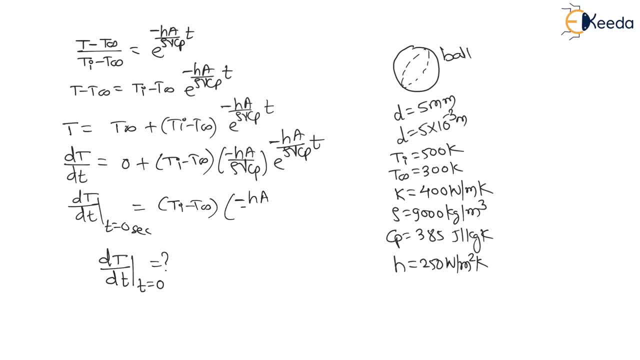 T infinity into minus H A, divided by rho, V, C, P. This will be our resulting expression. So let us solve this equation Now, my dear students here, your answer will be: the area of sphere is. we know that 4 pi r square area of sphere. 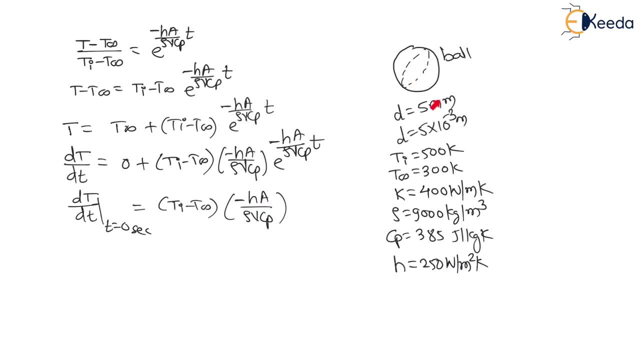 which is available for convention is 4 pi r. square Volume of sphere is 4 by 3 pi r cube. So, my dear students, let us find this area. We have a volume ratio for sphere. Area is 4 pi r. square Volume is: 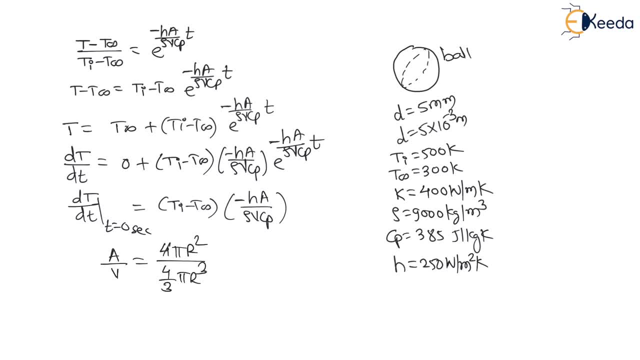 4 by 3 pi r cube Now here: 4, 4 pi pi will get cancelled. r square, r square will get cancelled. The answer will be 3 by r, which we can write, 6 by d, which we can write 6 by d. 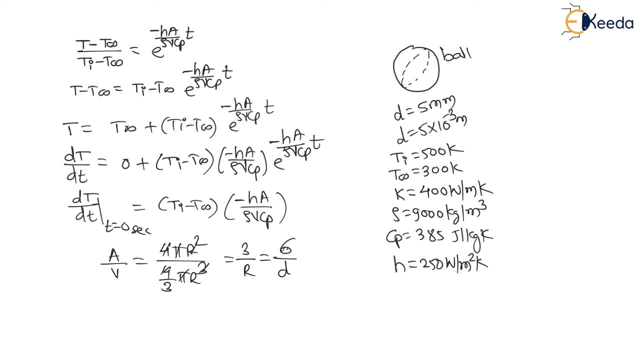 So let us replace here area- we have a volume- with 6 by d, because dimension of this sphere we have right. So the resulting equation becomes: DT by DT. change in temperature with respect to time. that is, change in temperature DT by with respect to time, when your time 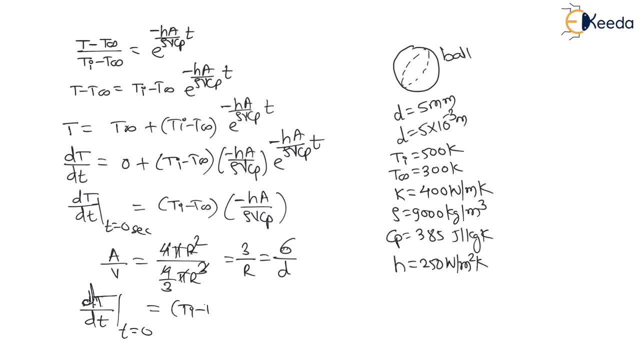 is equal to 0 will be TI minus T, infinity, into minus H, into 6 by D, into rho CP Area divided by volume- here I am replacing with 6 divided by DP diameter. right? So, my dear students, let us put the values here. 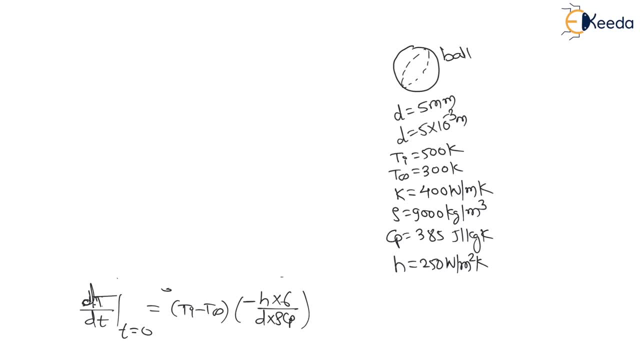 right Here. let us put the values. Therefore, I will get this: DT by DT, DT by DT, when your time is equal to 0, is equal to initial temperature. TI is 500 Kelvin. the T infinity surrounding fluid temperature is 300 Kelvin. into minus. H is nothing but.